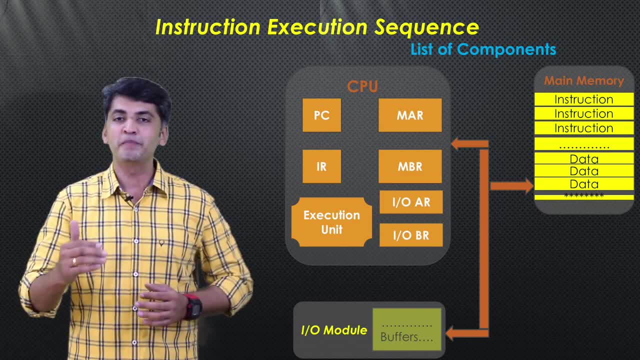 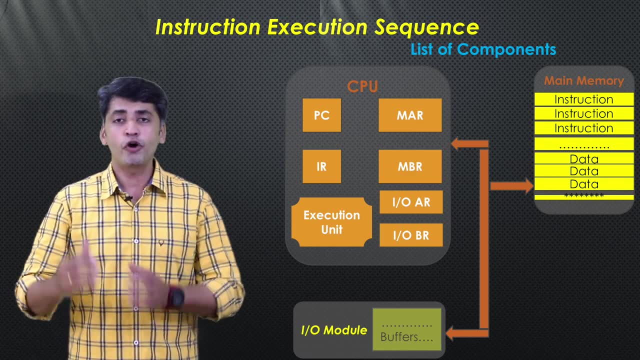 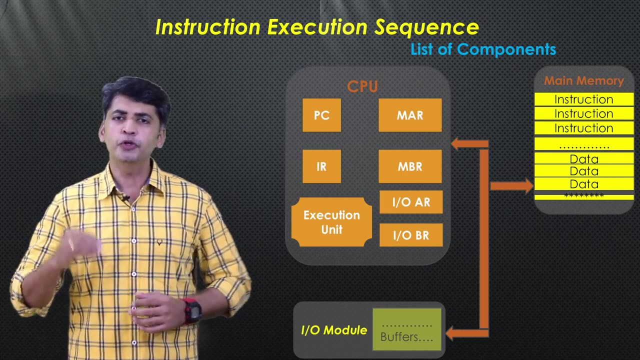 is a memory address register, and the third one is MBR, that is a memory buffer register, and the fourth one is IR, that is an instruction register. so after that IOAR, that is an input output address register, Then I O B? R is input output buffer register and last one is the execution unit. So these are the 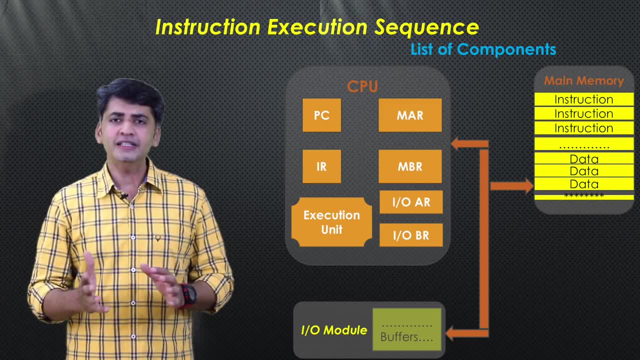 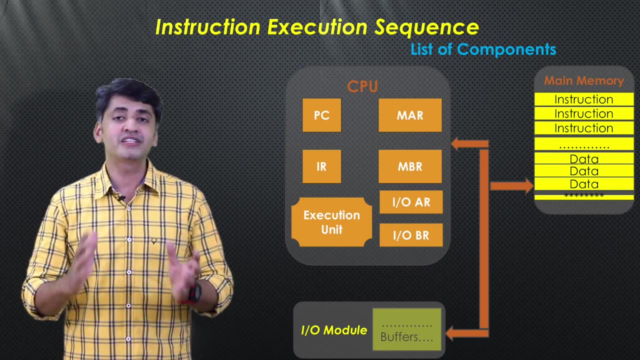 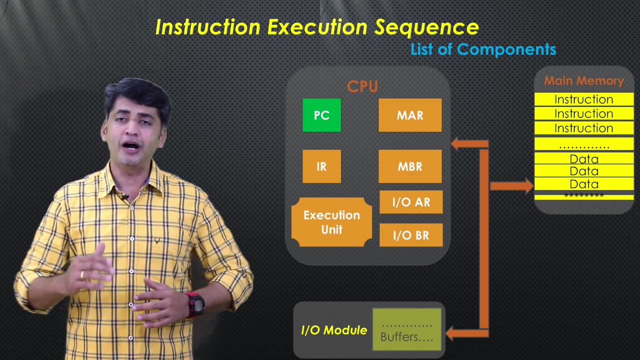 major components inside the CPU. After all these components, two other components are there, These two components associated with the CPU for this instruction execution. One is the main memory. second one is the I-O model. so we'll see the functionality of the components. 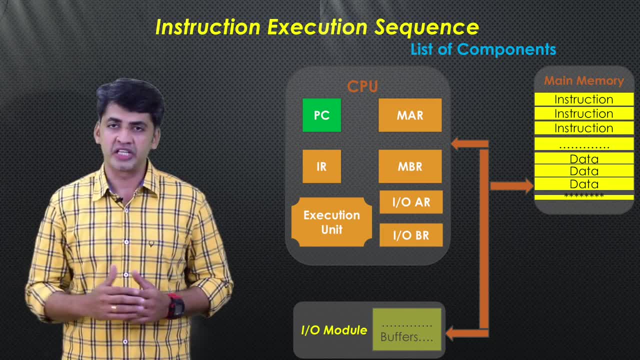 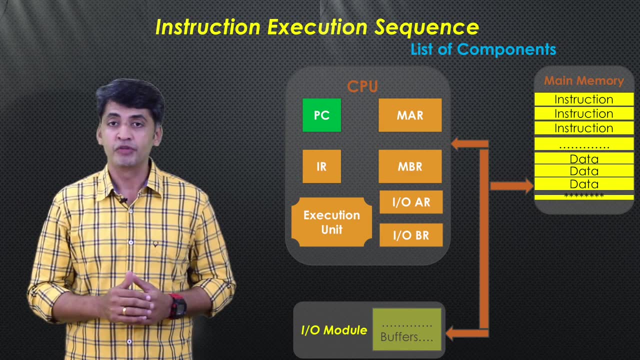 after that we'll start discussing about the instruction execution sequence. the program counter that is a PC, so it will store the address value of next instruction to be executed. so example: you just consider if the program is going to be executed, the first instruction address will be there in the 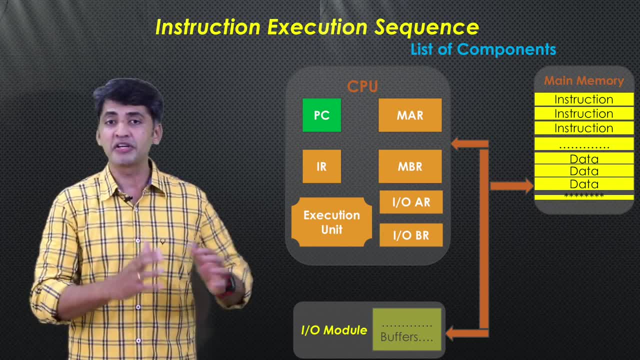 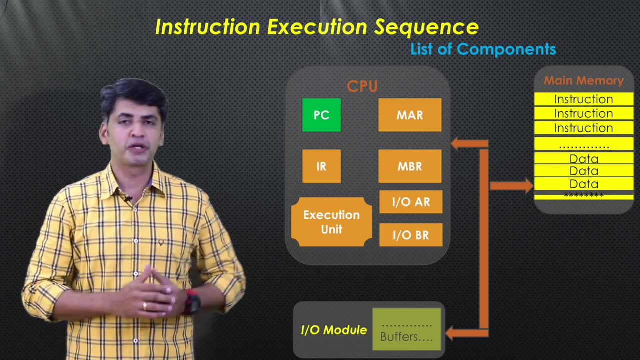 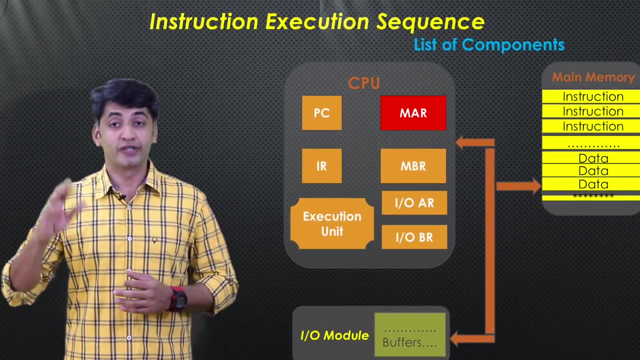 program counter. so after instruction, after the program execution starts, the next instruction value will be address value will be there in the program counter. so this is the need for program counter. and this next one is the memory address register. so this will be used to store the value of address for the 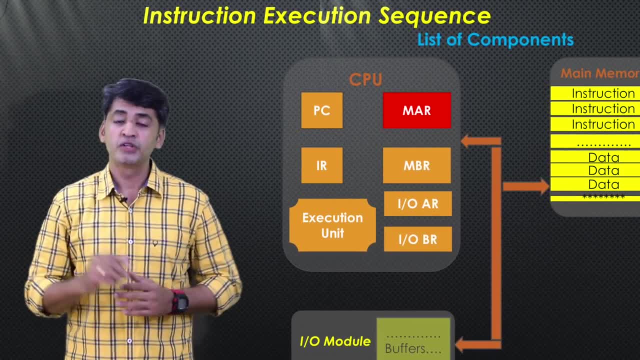 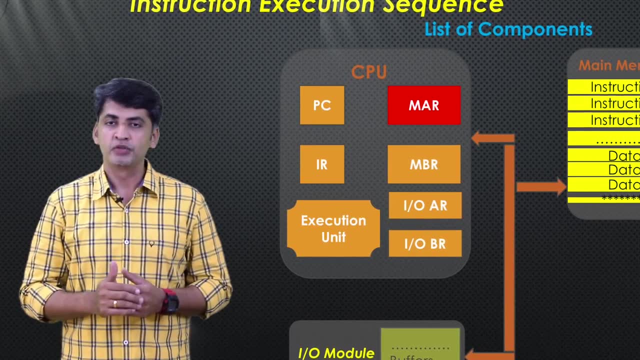 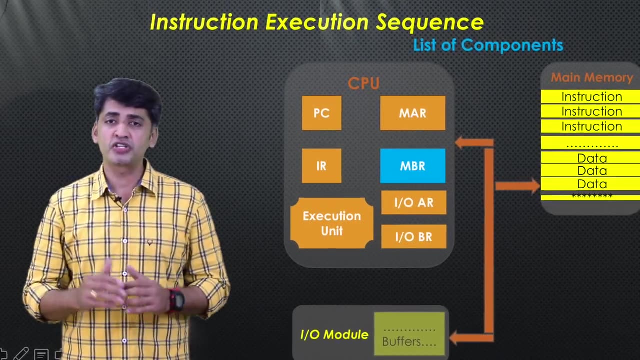 address calculation. so here address value will be stored here so it will be used to identify the exact location in the memory that address value can be stored here for the data transfer and data store. and next one is a memory buffer register. so this buffer register used to transfer the data between 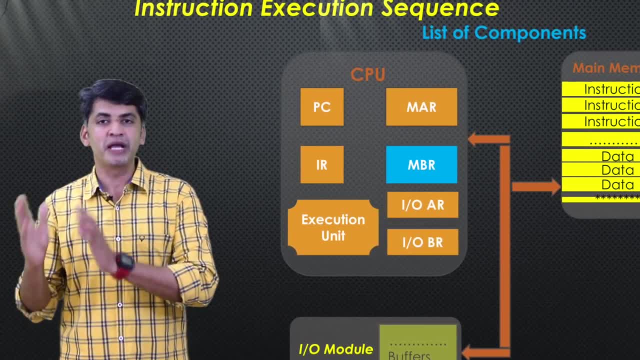 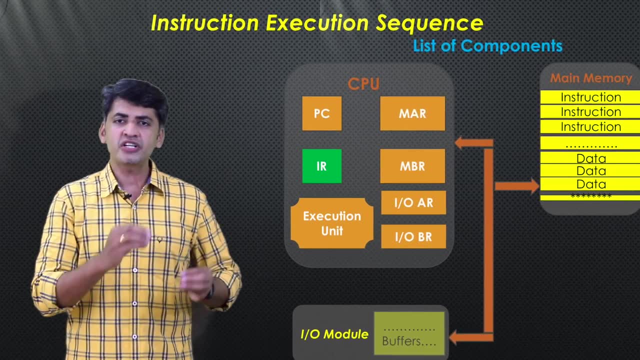 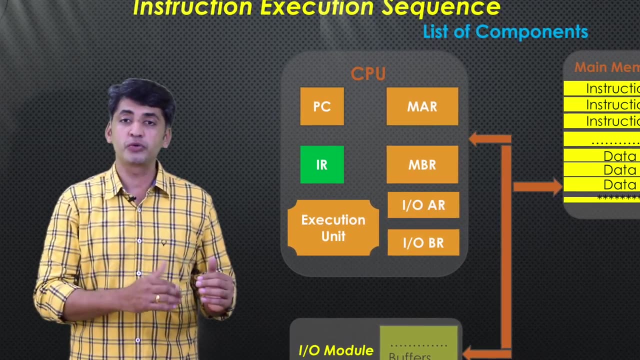 central processing unit to main memory and same time main memory to central processing unit. so this is the need of MBR. and next one is the instruction register. so instruction register means it will be used to store the instruction, so for the execution purpose, so before the execution, so instruction will be stored in the 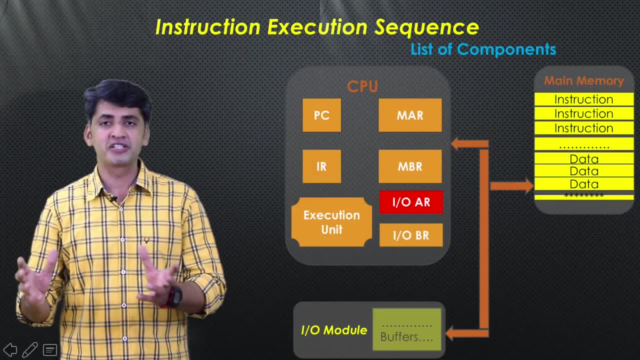 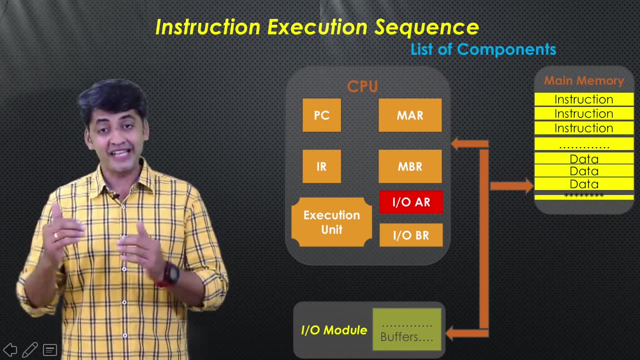 instruction register. so after that: I-O-A-R- that is a name itself, it's the meaning is there. that is input output address register. so for the I-O model. so this address register will be used same time. I-O-B-R. so that is the input output buffer register for the I-O model and the 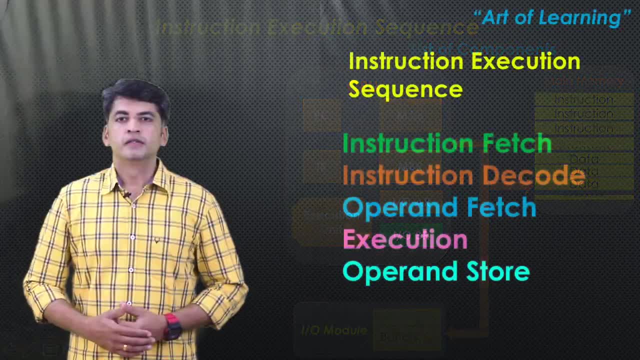 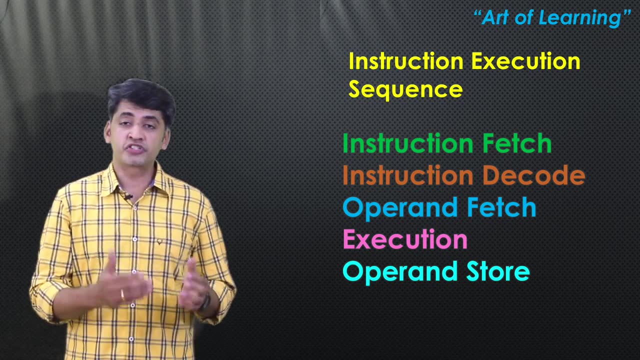 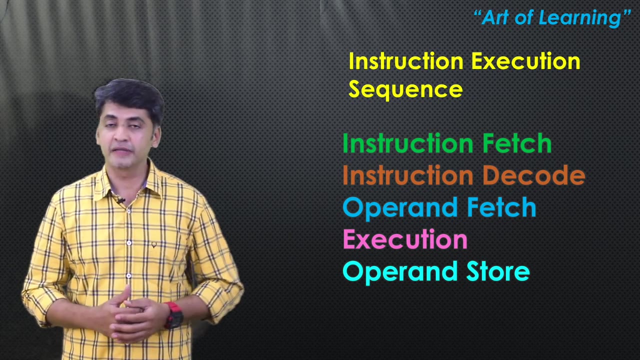 CPU data transfer. this buffer register will be used for the instruction execution sequence. the first step will be the instruction fetch and second step will be the instruction decode, and third one is a operand fetch and the fourth one is the execution, and the fifth step is the operand store. so we'll see one by. 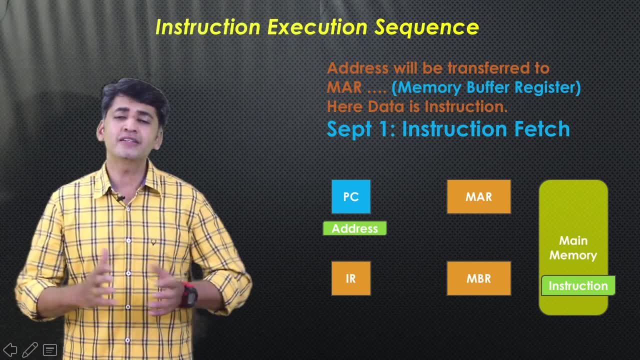 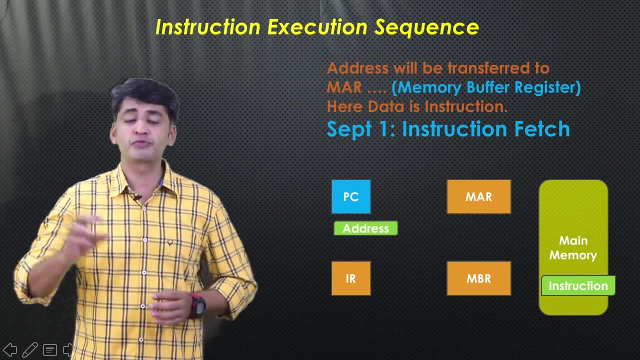 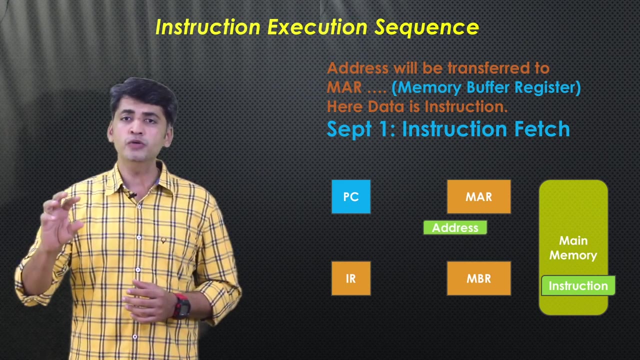 one. the first step is the instruction fetch. so during this instruction fetch, so program counter will have the address value of the instruction. so that address value will be transferred to the M-A-R, that is, memory address register. so what is the value will be there in the memory address register. so 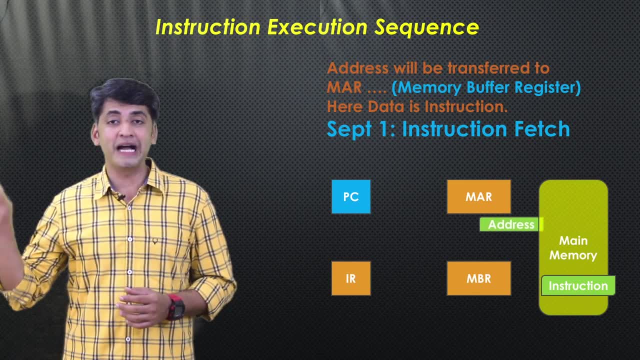 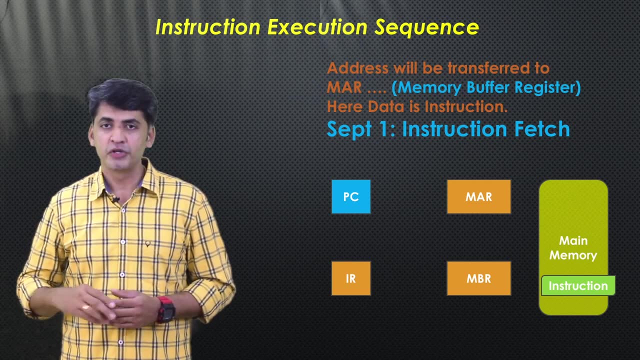 according to that memory address, the address location will be identified in the memory. so that memory location, the instruction will be there, so that instruction will be transferred to the MBR, or that功은 명, Maj Kou Roller, ほとんどのCLI updatmers Krug, 方法を改 ihren judgments will be transferred to the MBR. that is a. 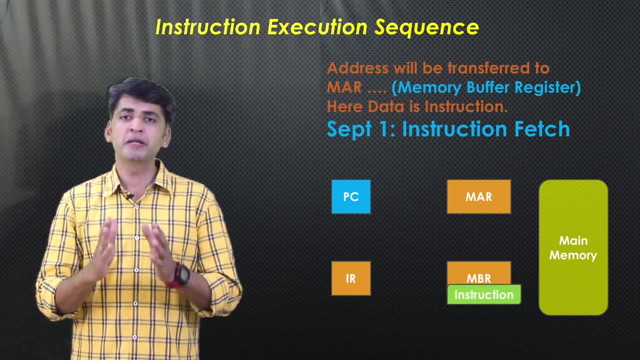 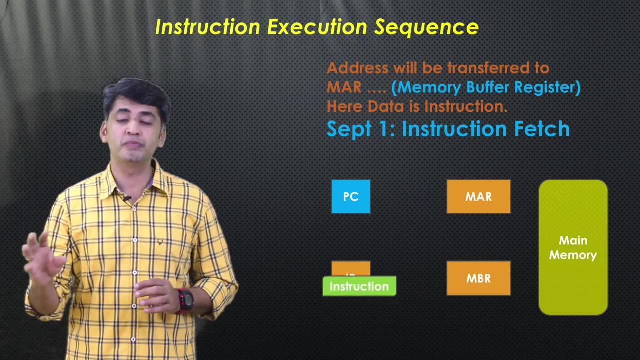 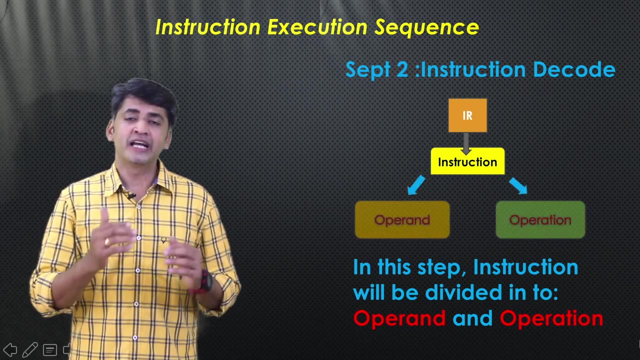 buffer register. So after that, from the memory buffer register the instruction will be transferred to the instruction register. So this is how the instruction will be fetched to the instruction register. This is the first step. The second step in the instruction execution sequence is instruction decode. So here: 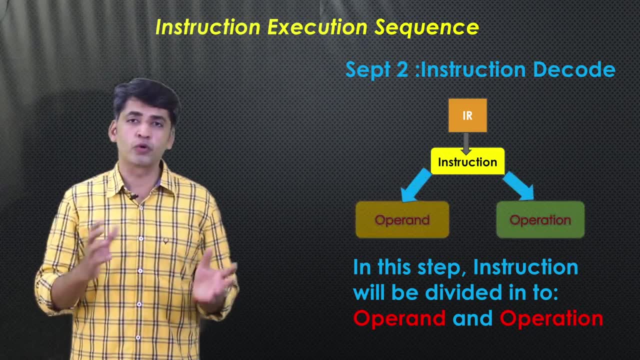 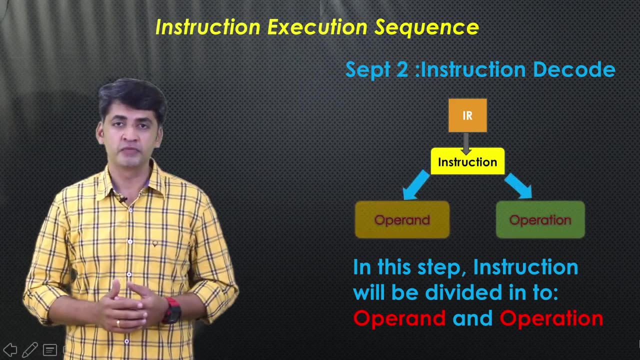 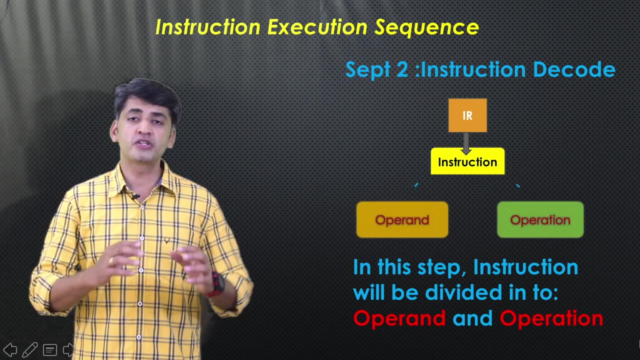 the instruction. the fetched instruction will be decoded and it will be divided into two major components: one is the operation and second one is the operand. So, based on the which operands, which operation will be executed by the execution unit. So this is how the instruction will be divided. that is, that is the meaning of decoded, and 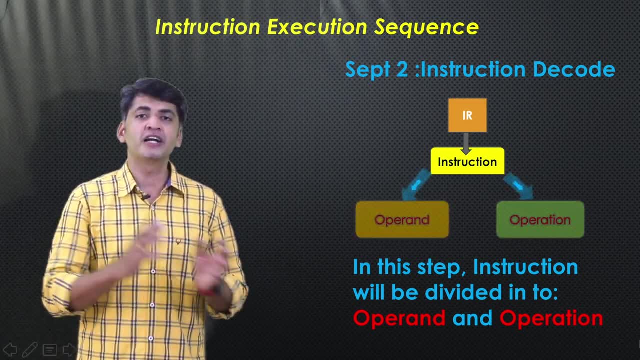 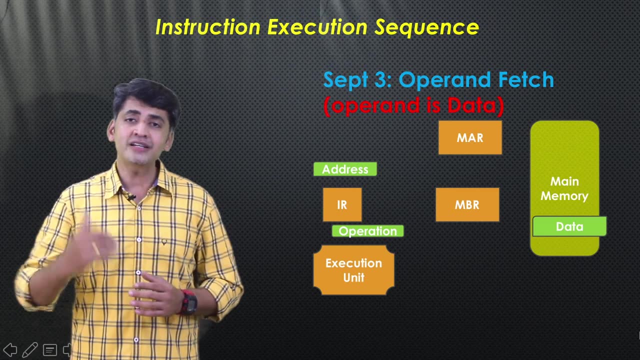 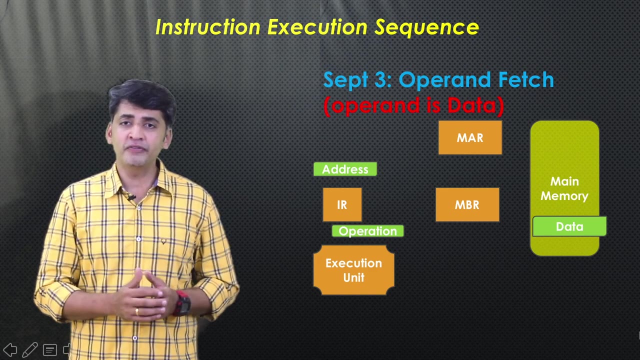 it will be find that which is the operation and which are the operands. So this is the second step in the instruction execution sequence and the third step is operand fetch. So here again the registers will come into the picture during the operand fetch. so the operation will be there. for that operation you need the operands. for that operands you. 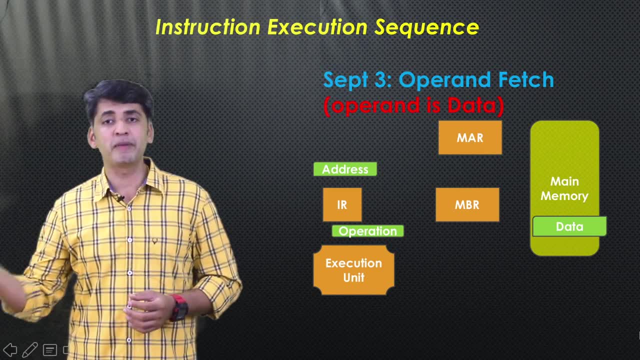 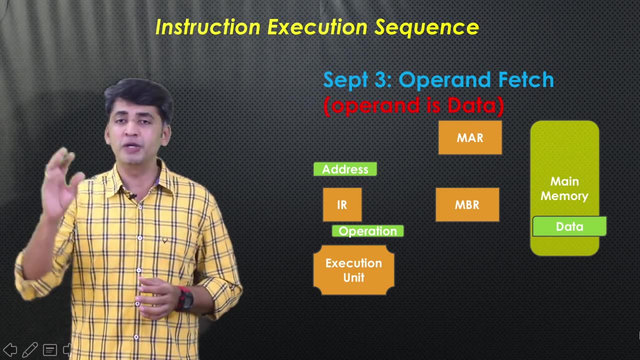 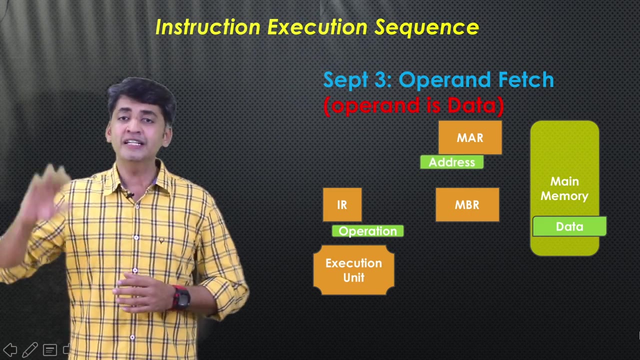 need to identify the memory location. from that memory location those operands will be transferred to the central processing unit. for that you need to calculate the address. that operand address will be passed to the memory address register. from the memory address register the address value will be identified.